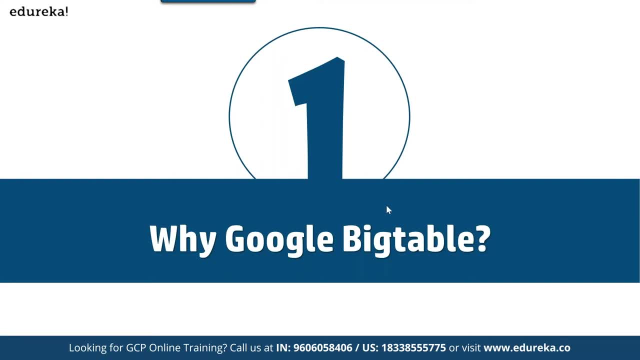 which is basically, you know, being provided by Google. So we are in. you know, Google is going to host your entire data on that platform. So you can do everything. you can create virtual machine, you can create database. any of the things that you can do at your on-premise platform can be done. 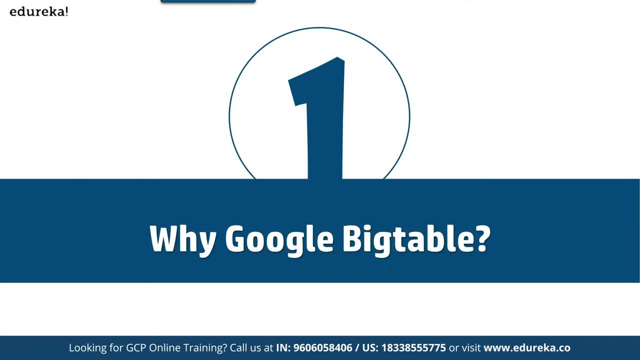 on the cloud at the safe of ease. At the same time, you can perform that integration with different tools, technologies that Google has very easily. So now let's talk about you know why Google Bigtable. Before we talk about you know why Google Bigtable, What is the use case of it? 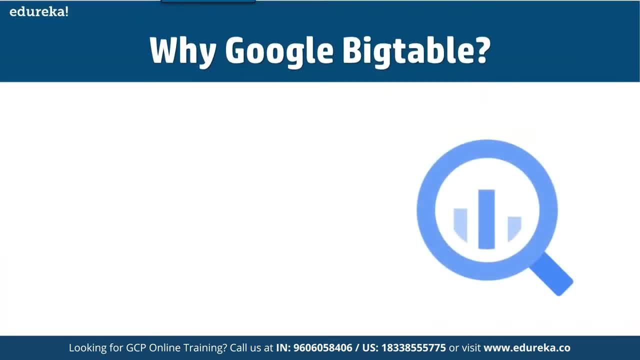 Why exactly we should use Google Bigtable. These are a couple of advantages. So it has unique data warehouse services. So your data is going to be, you know it's going to be, you know, kept at various locations, various places. So it has a unique data warehouse services. It's not. 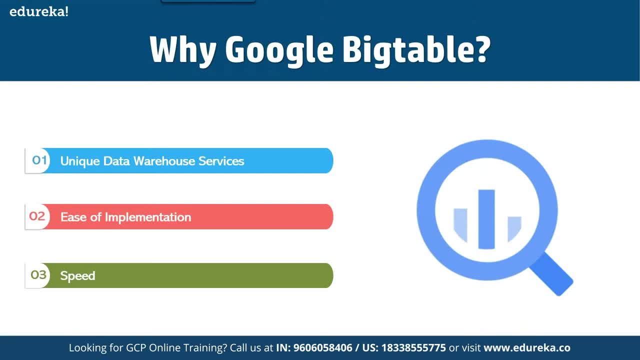 like that. you know, at the same one data center you're accumulating all the data for all the customers, So it basically provides you high availability And at the same time it has the unique services for each of the user. Second is ease of implementation. To work on this is very. 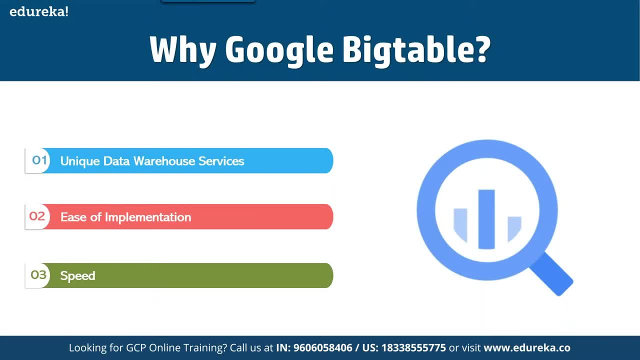 easy. Some people think that oh, it's a cloud, so it's very difficult for you to use and implement. We have to. you know, say we get a network, it's going to be very complex. So once you're going to, 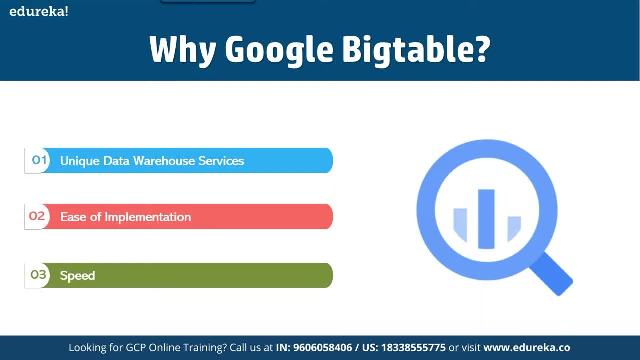 work on it. you're going to have a lot of data, So you're going to have a lot of data, So you're going to see the interface. You're going to get an opportunity to work on this and dive in more detail. You will see. it's very easy. Plus the speed, It's very fast. Now, for example, you are 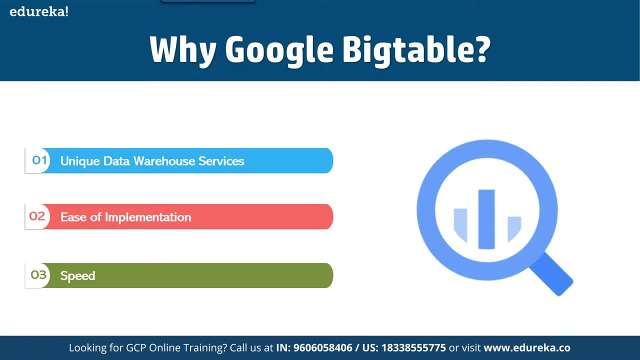 going to create the resources. Let me, you know, give you a very small example. I have to install an operating system on my laptop. How much time it takes. Approximately an hour, right? Or if I have to also, let's say you know, create a virtual machine on my system, it will take how? 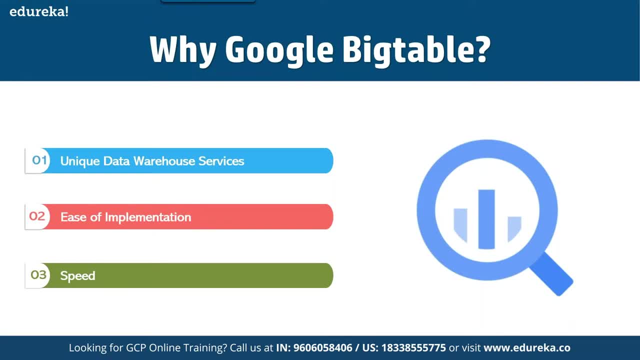 much time- Approximately an hour- Here in the case of Google GCP platform, you can spin a lot of resources in. you know, less than five minutes. If I had to create a virtual machine, less than five minutes I can create it all And you know it's not going to be an issue. 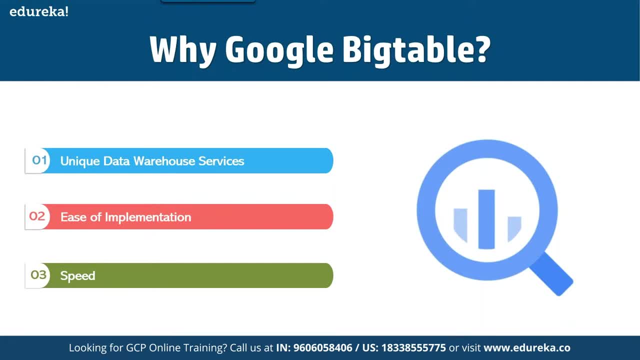 So, at the same time, it's going to provide high availability as well. If my data is going to be lost, like, let's say, if my, you know where I hosted my data, like in my on-premise environment at my data center- if the data center goes down, my entire data will go down, right. However, in 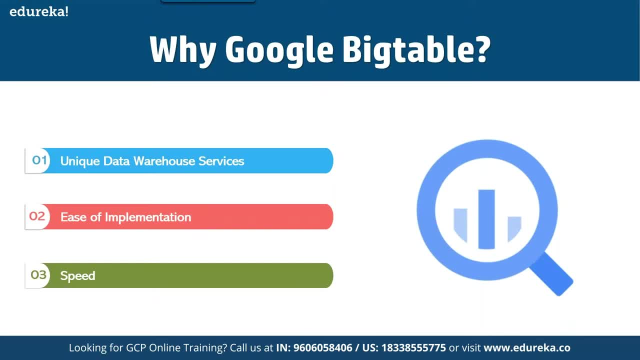 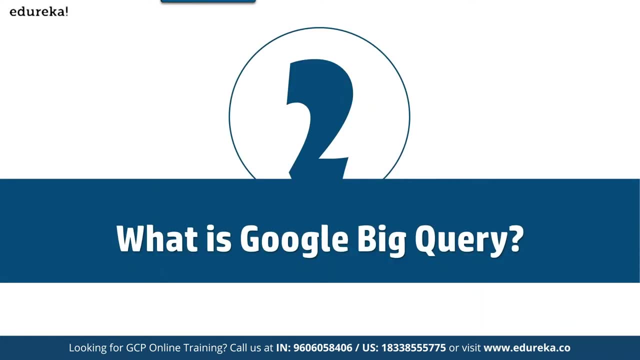 this case, that's not the case. If your primary data center is down, it's going to perform automatic replication. So it's not going to be able to do that. So it's going to be able to do that. So data is going to be replicated very easily. Now, what is Google BigQuery? Let's 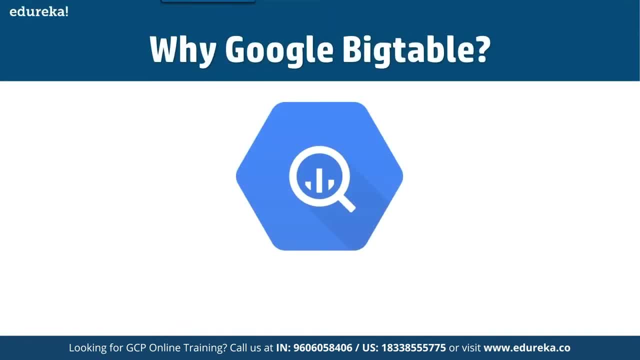 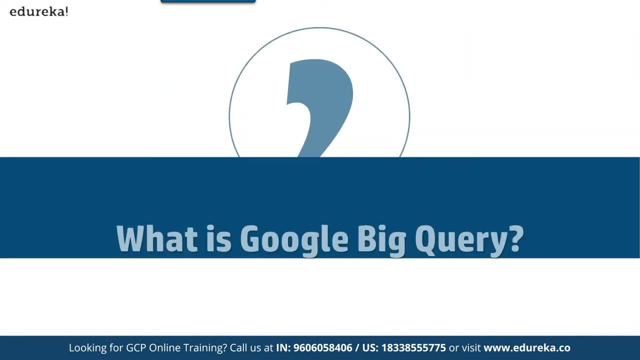 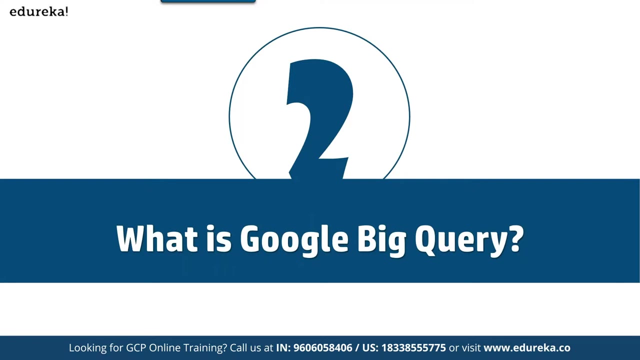 just get understanding of it. So before that, you know, let's understand Google, BigTable and BigQuery. So basically, BigQuery now we're talking about. you know this guy. So basically, your BigQuery is a fully managed, serverless data warehouse service that enables scalable analysis. 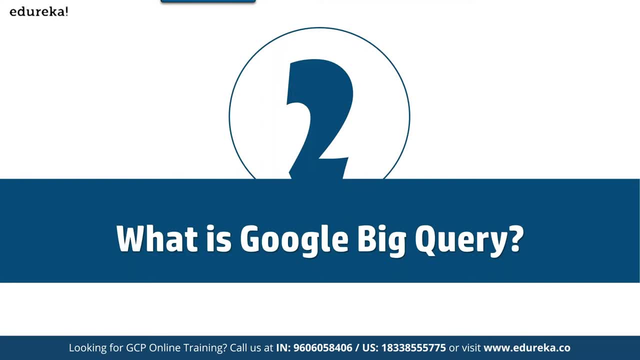 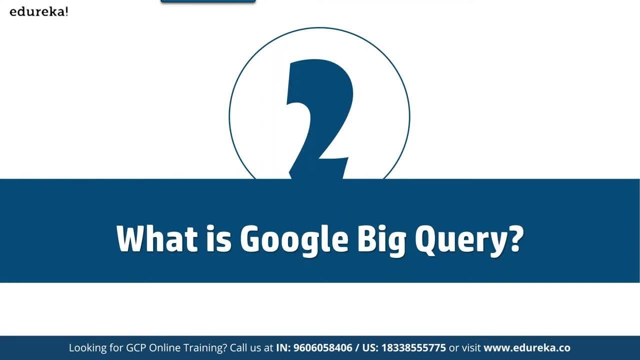 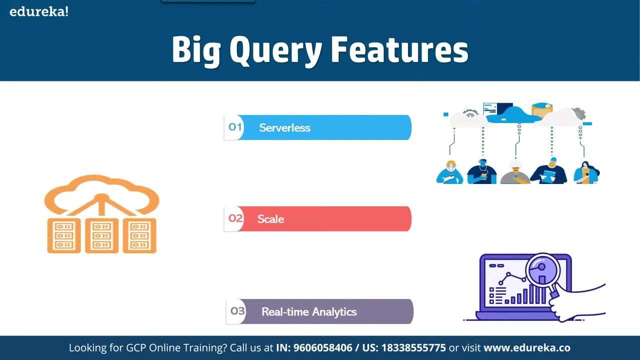 store the data in a large storage and whatever you're going to consume, you're going to pay for it. Now, what are the different features of it? Now, coming to different features, it has various features like: first is serverless. What serverless means? It means that in order to run this, 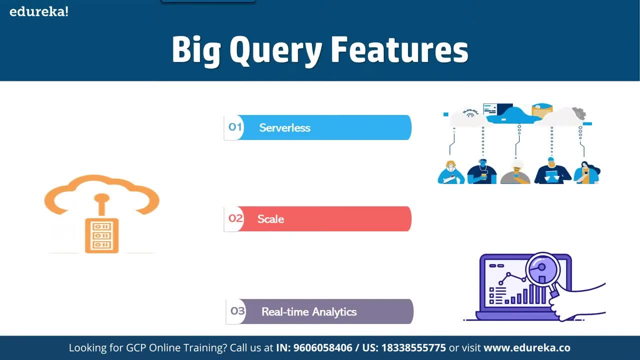 there is no dedicated server required. Now you know that if I had to basically run the resource support I will need, I will need a resource, a virtual machine, basically that way that I will require to run those resources. right, So it's a serverless. You don't require the server without. 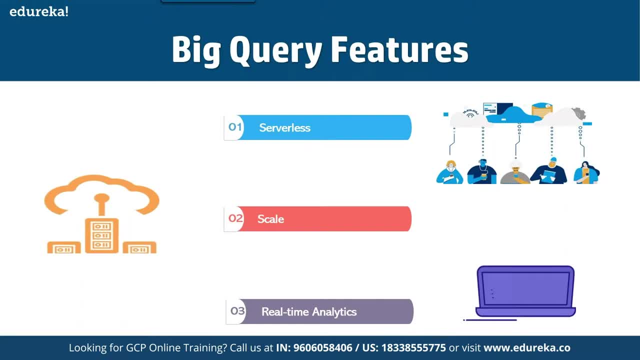 having the server, You basically can, you know, deploy your resources, You can access it, You can integrate with the application Plus, since you are not going to use a server. so having that overhead to manage the server, performing the patching, installing the updates, you know. 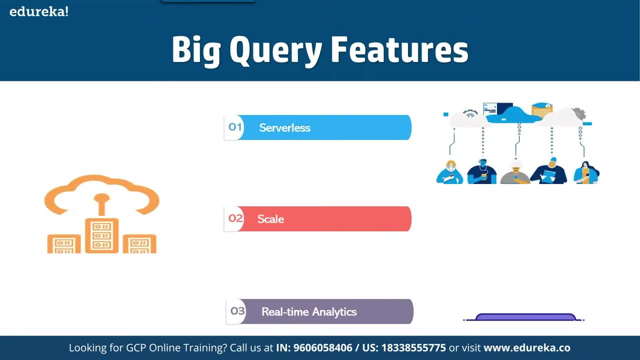 even paying for that dedicated environment. you can just save the money on that. Second is scale. So it basically you can perform the scaling as well. You can basically perform automatic scaling at the same time. You know it's basically supports petabyte of data. So if you want to, 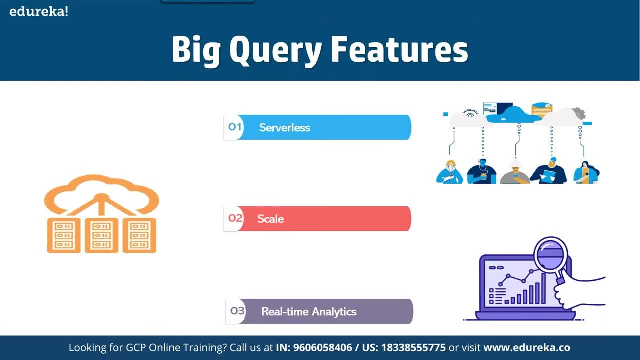 basically scale with, let's say, you know more CPU, more RAM, then you can do it very easily with this. In addition to that, in addition to scaling, let's say you want to increase number of code processors as well, you can do If you want. you can write a script, you can write the. 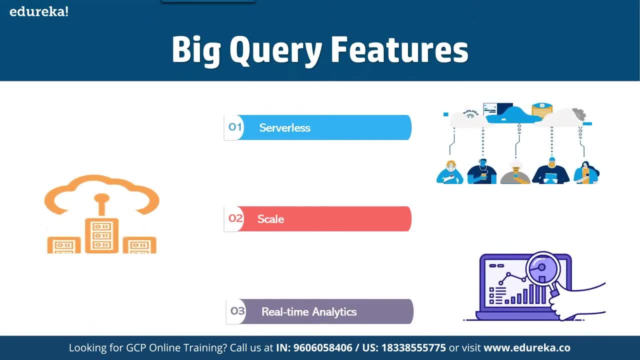 criteria, For example, if your CPU utilization is going to go high at a certain with a certain. So in that case, in such kind of scenario, what you can do is it's going to automatically increase the resources When the CPU utilization is going to go low, it's going to automatically. 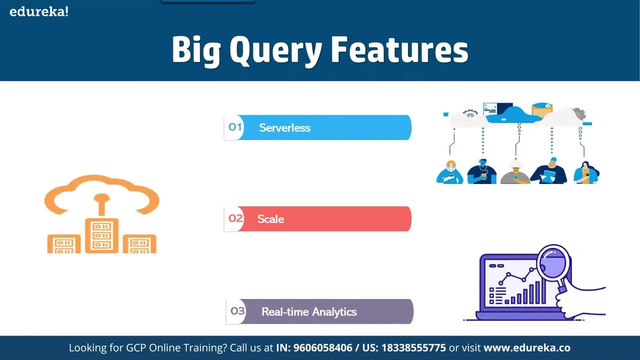 decrease the resources. Next is real-time analytics, So wherein you can basically inject the data from various sources. in this And, as you can see here, towards the right, you can see the progress. Like I want to see my company's going in profit, My company is going in loss, but each 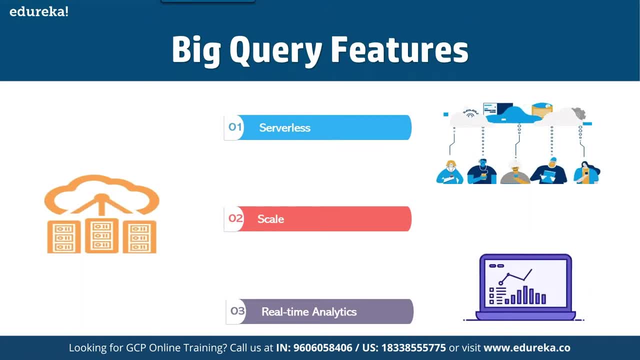 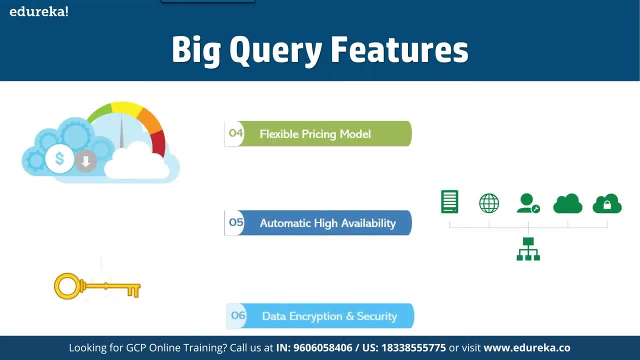 and every information at the stake of fees. it's going to be available and you can get the information very, very easy Now. next one is your flexible pricing model. So in fact, you go to believe it's type of pricing model that we have. one would I have. 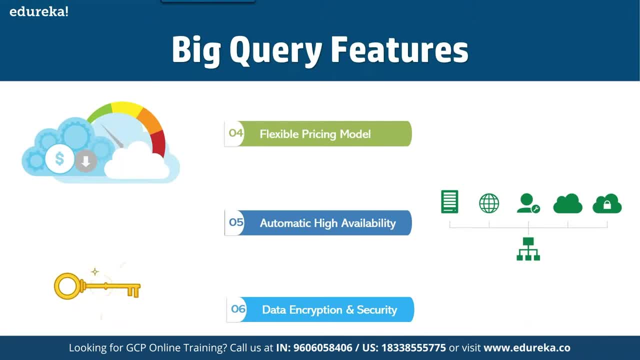 more detail today. So it supports flexible pricing model. We, if you can uh easily get the, I would say you can easily pick up the package depending on your need, depending on your requirement And addition to that, you have to. also, you know you've got investment aside all over. 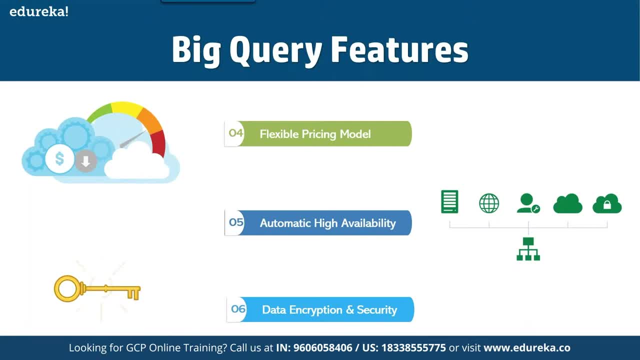 the monthly package, Yearly package. I won't do the services the way the services i'm going to do, so that's something. uh, you'll be able to have that entire- uh you know, flexibility with this. plus you have automatic high availability, so whenever you, 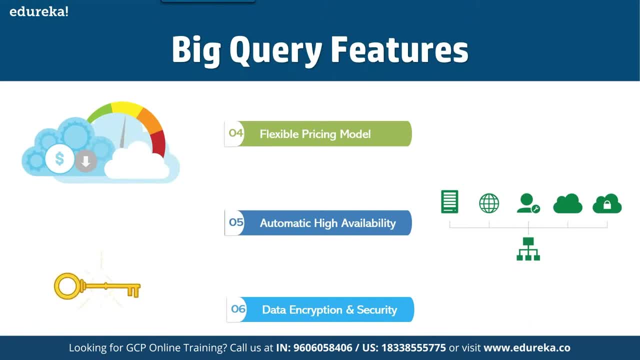 are going to create the resources. uh, in this case, in the case of bigger, google, bigquery, those resources, basically, are going to be, um, you know, replicated at the different sites, depending on the site model that you're going to use. those resources are going to uh be, you know, replicated. 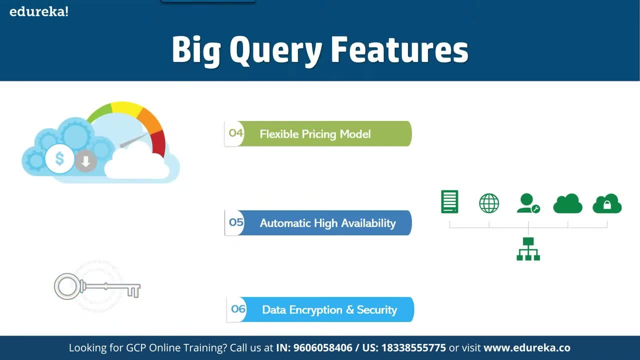 automatically. at the same time, it also supports data encryption and security. so you know that nowadays, encryption is one of the biggest requirement. based on the ongoing hacks- uh, so many companies were hit by the ransomware as well. so, in the case of data encryption, what happened is your data is going to be encrypted automatically with the key and that key you can. 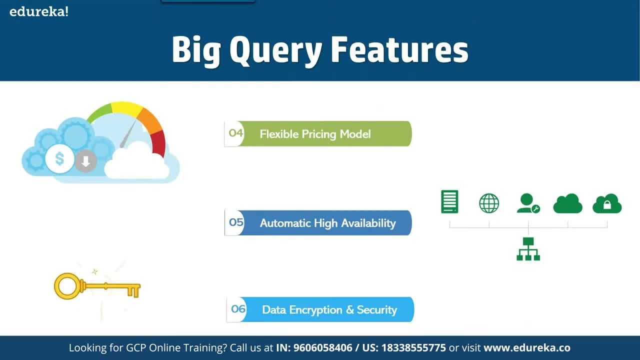 store in a keyword in hsm, depending on the requirement that you have. so that also provides- and now, if i talk about the security, it basically supports. uh, you know our back as well, which is role based access, where in you can basically define that. uh, you know like which user which, what kind of role you. 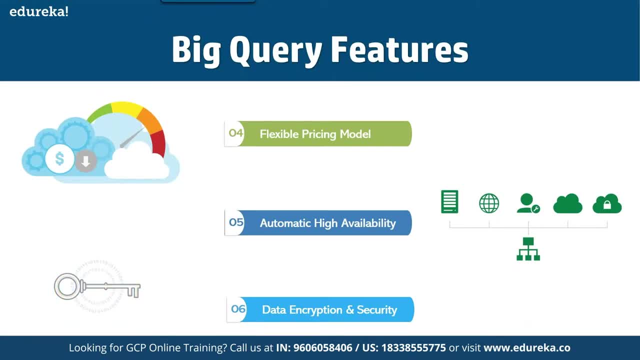 want to assign. so all those, those things, basically, are available here as well, and the sake of this, plus, there's no, uh, you know, specific, uh complex, uh implementation. each and everything is designed in such a way that you can get, uh, you know, easy interface with easy integrations as well. you can. 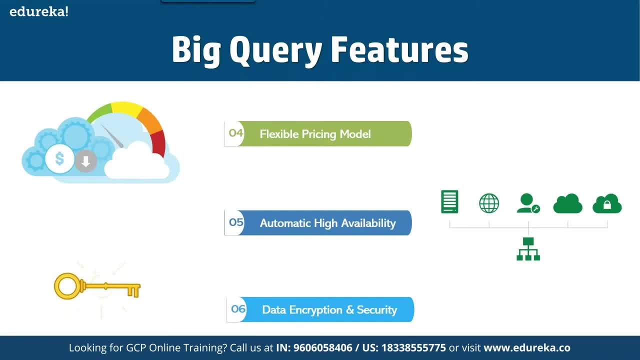 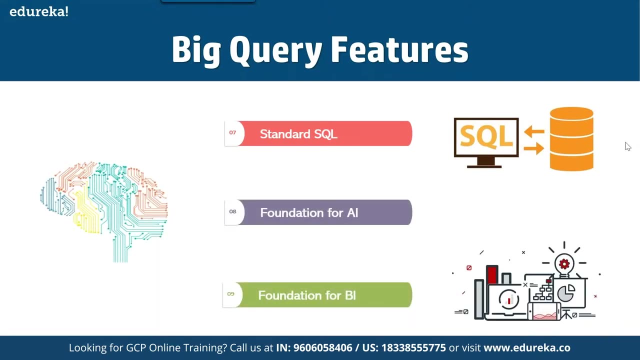 make a api call using different programming languages like java, python. different apis are also available. you just have to change the you know some variables over there and you will be able to use it directly. next one is standard sql, so it automatically have inbuilt standard sql, uh, at the same time, you can also- uh, you know- define your own database. 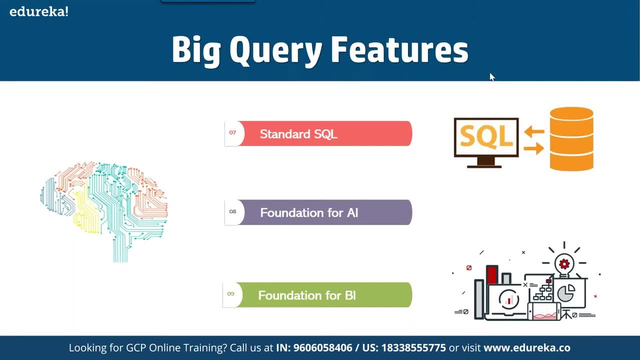 by, you know, creating a new resource in that you can also create your own database as well. next is foundation of ai, which is artificial intelligence. you can integrate with uh- you know our different images as well- and you can also integrate with dia as well, which is business. 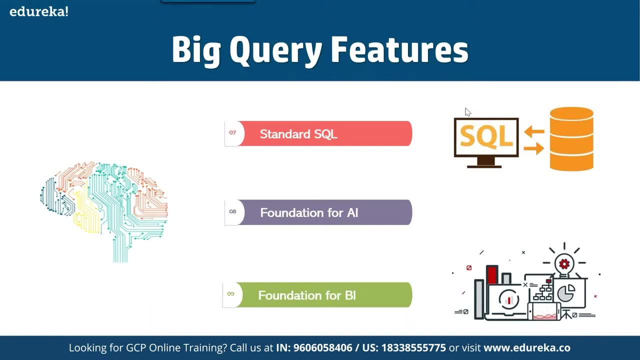 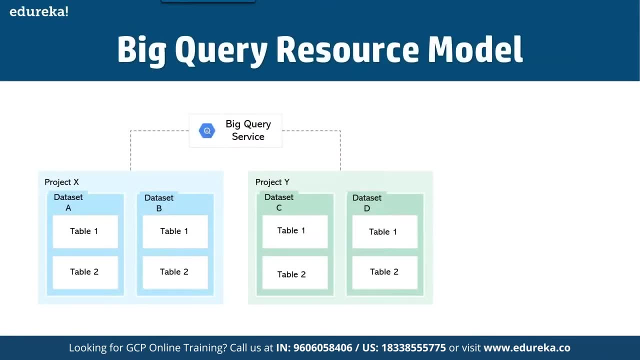 intelligence. yeah, now moving on, let's talk about the big query storage. so in the case of big query source model, it basically have five major components: the projects, the data set, your tables, your views and the jobs. now here, in this case, let me just use this highlighter. you know, this is a project. basically, one project is foundry in that project. 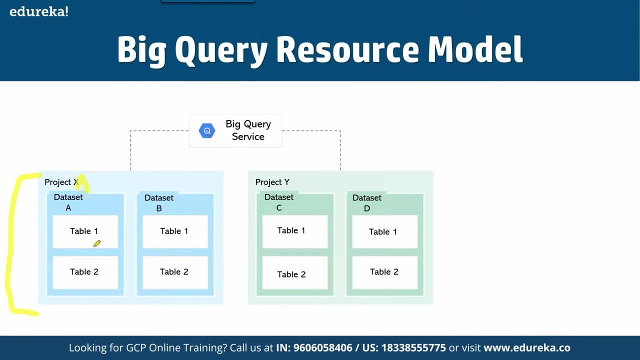 basically you have a data set. in that data set, you can basically have, you know, a couple of tables. so now in those tables, you basically can have different views and you can basically, you know, have different jobs. or now this is a different project, now likewise you can have different. 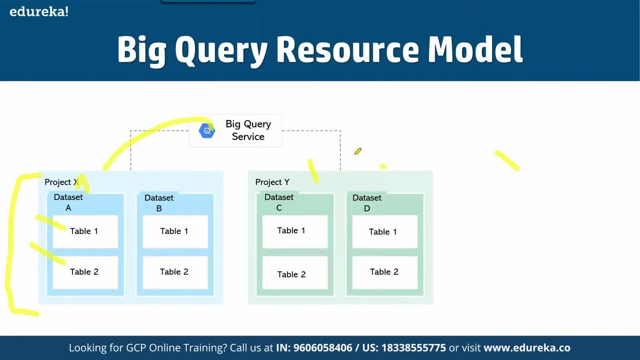 different projects here which can be integrated directly with your bqs, which is bigquery service, wherein you can easily- you know- query the data. for example, this project needs some data with you know this project or this project needs it with this project, or some different project needs. 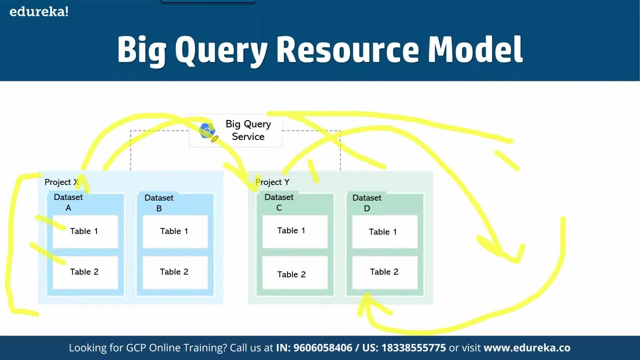 your data with this project. so this entire management, that role basis control, can be easily to be used and run in big terms for big annreal projects. presence control can be easily be done with your big uh my database control and then you have also uh azure data set priorities. this project is a different things. I'm sure they can have some of this uh things, but for this one, this project, or some different things, while I'm 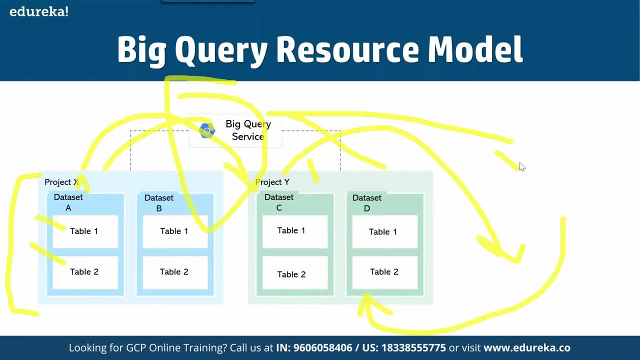 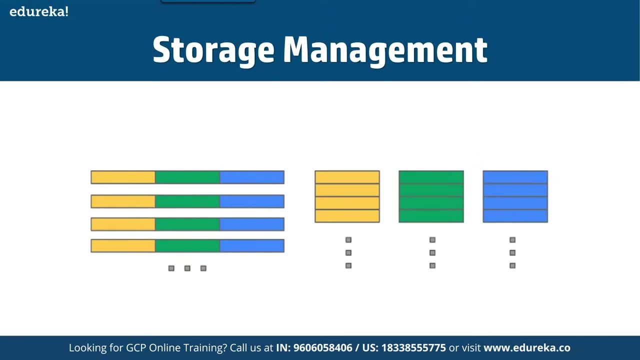 BigQuery service. So that's again a little bit over here at a higher level. Now, coming to the storage management that we have, let's take a look at how storage management looks like of BigQuery and how it is different from others. So this is towards the left. you can see this is traditional. 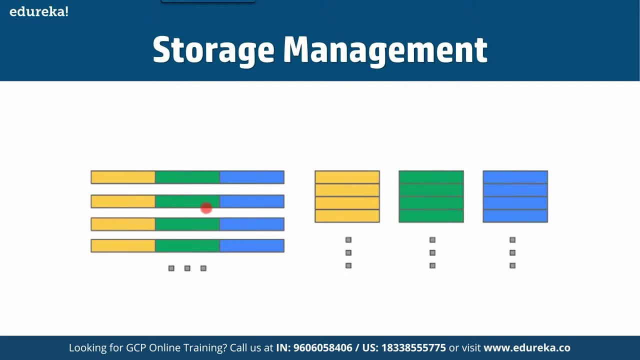 RDA, BMS storage, where you are going to have record-oriented storage Like this is the one record, second record, third record: likewise On the right side. you see this is BigQuery storage. So here it uses the column-level storage. Now, even if I want to perform encryption, 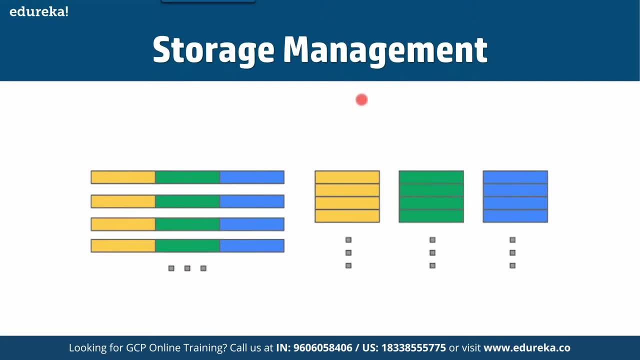 I can perform encryption in one column, Maybe I have a data. let's say, in one column I have name. second column I have their last name. third column I have their credit card number. Now this blue one is sensitive for me, But if I go with the traditional RDA BMS storage, I have to basically 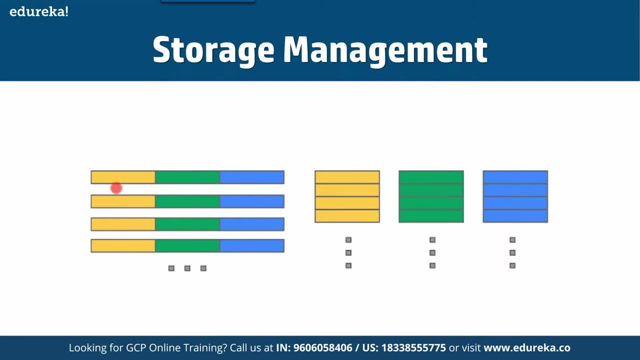 encrypt the entire row. It's going to be difficult for me And, at the same time, encryption, decryption will take time. The operations execution will take time, which is going to be difficult. Now towards the right, if you talk about, you know, BigQuery storage, we are going to have the 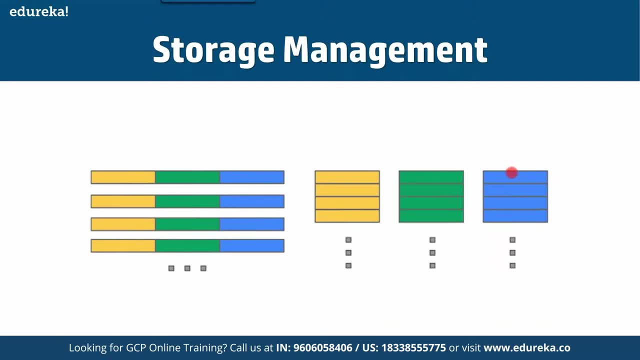 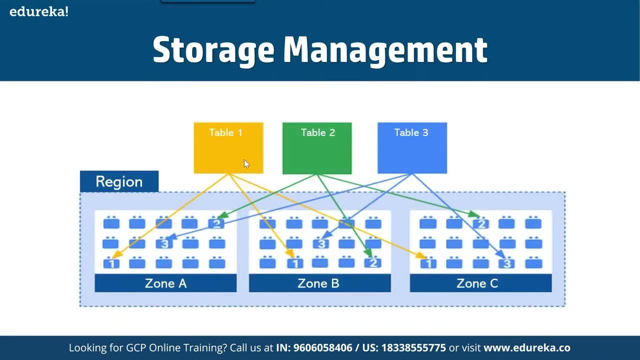 column-level storage, where we are going to encrypt one column at the time. Now coming to the other one, which is storage management. Now here, in this case, as you can see, like we have this table one, table two, table three, In one region, we can have different zones, Different zones, basically like 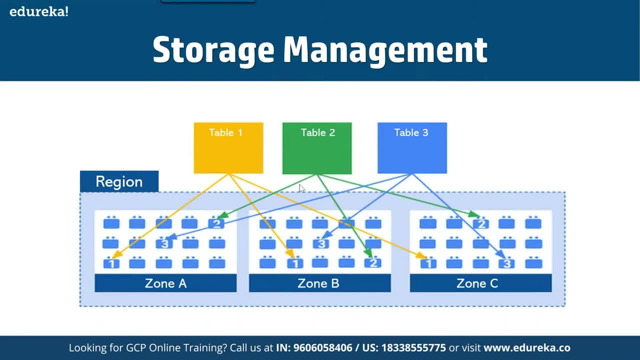 your different data center. Maybe in India? I have this data center in Bangalore, second is Hyderabad, third is Delhi. So if one zone is down, we can have a different data center. So if one zone is down, we can have a different data center. So if one zone is down, we can have a different data center. So if 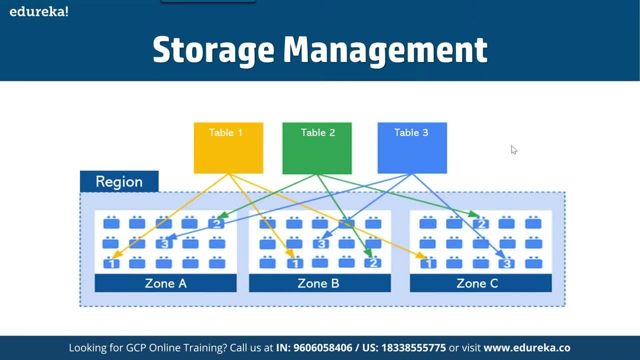 my data is still going to be there at the second, at the third, Now here. in this case, if you see, this second one is available here as well, It's available here as well, It's available here as well. So the same data from table two is pointing out to this, The same data is copied at the second. 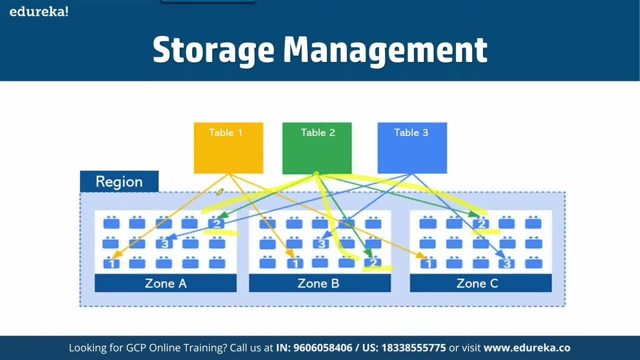 zone, Same data is also copied at the third zone. So even and similar in this table one. this is copied in the first, this is copied here in the second. this is copied here in the third, which is this one, this one. 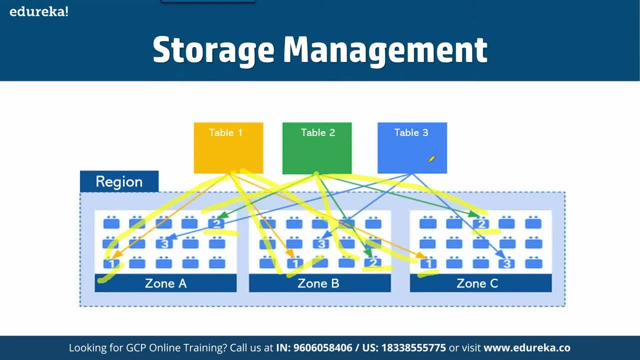 and this one. Now, in the third table, the same data you can see is copied here as well. It's copied here as well. It's copied here as well. Now, if this one zone is going to go down, this is going to remain up. This is going to remain up. Let's say, this one also got down. 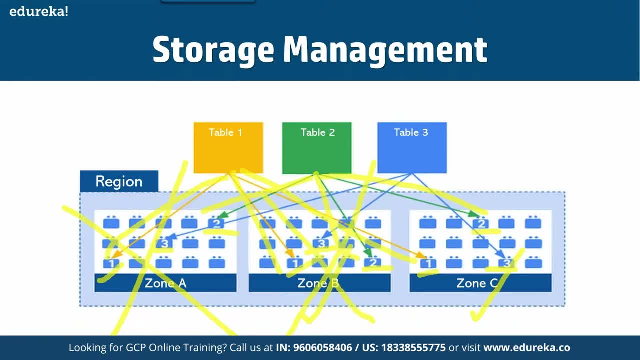 There was a network issue, So in that case, the third zone will remain up. Now you can have multi-regions as well, wherein the data from one region is going to be copied to the other region as well, So that's why it basically provides you a very 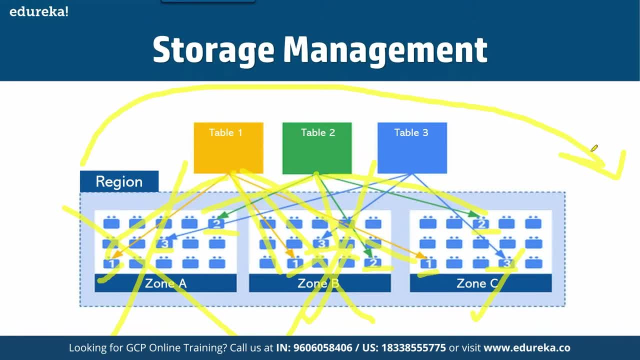 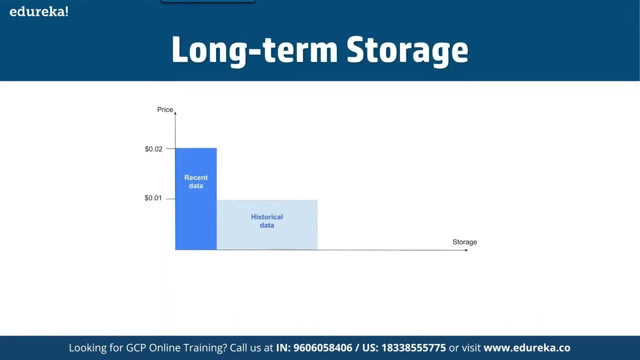 good resiliency and the data is going to be replicated automatically with the other data at the sake of ease. Now coming to LTS, which is long-term storage. So if you have a table or partition which is not modified for 90 consecutive days, it is considered as 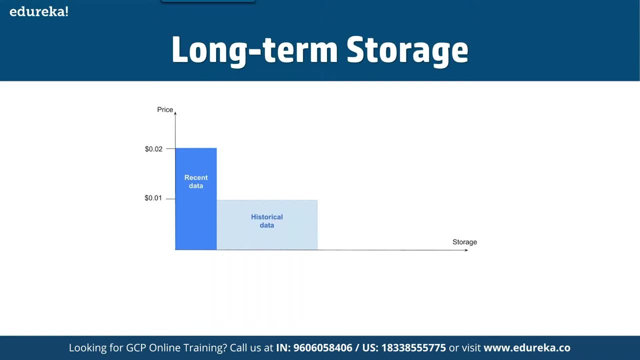 long-term storage And for pricing for the storage for that table automatically gets dropped by 50% to the same cost as cloud storage in airline. So basically, discounting is going to be applied on per table, per partition basis. That's the biggest beauty of it. 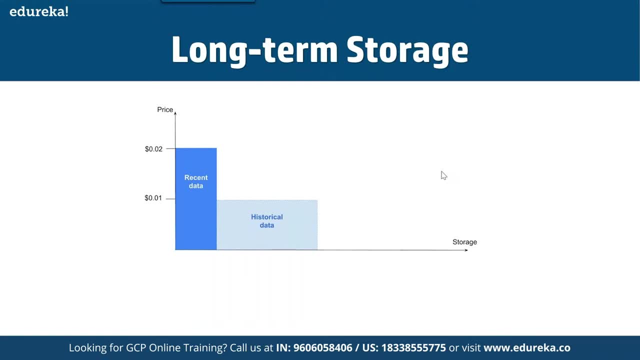 So if you're not using it, there is no need. there is no requirement that you have to change the storage type. It's automatically going to drop the price by 50% at the same cost. That's the biggest beauty of the Google Cloud, if I would say so, that you're not spending a lot of. 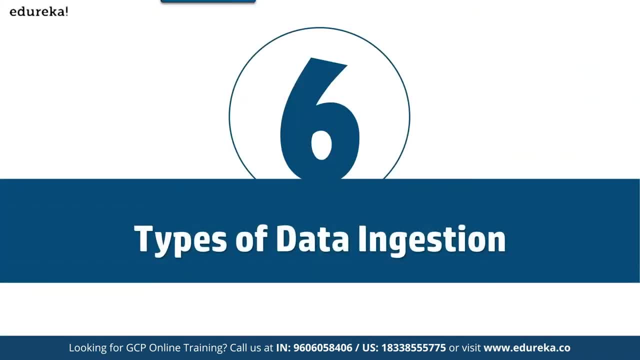 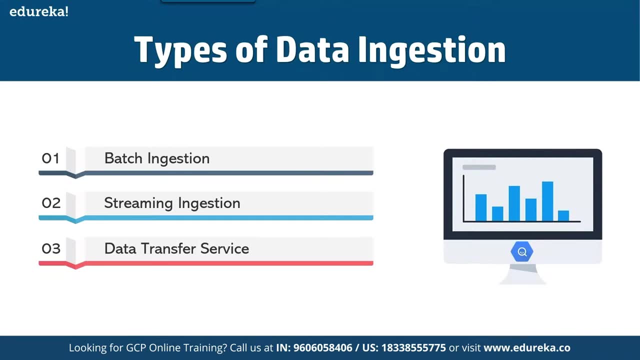 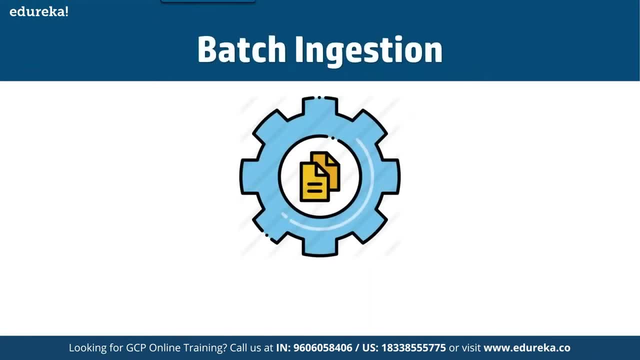 one by one. What is the batch ingestion? So batch ingestion basically involves loading pages, basically having a data set that does not have to be processed in the real time, So they are typically ingested at a specific regular frequencies and all the data which is going to 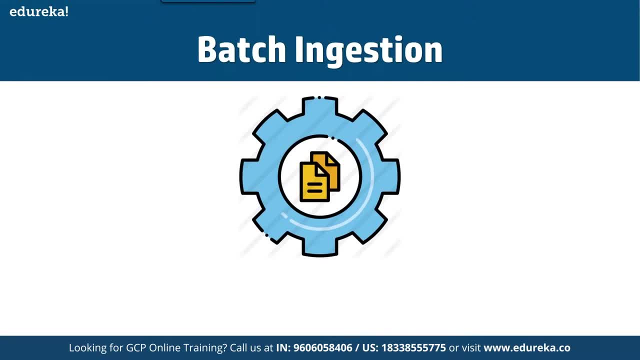 arrive. it's going to arrive at one time or it's not going to arrive at all. So the ingested data is going to be gathered on the on-premise platform and it's going to be processed together. So the batch ingestion is basically a little bit different. you know, you have data from 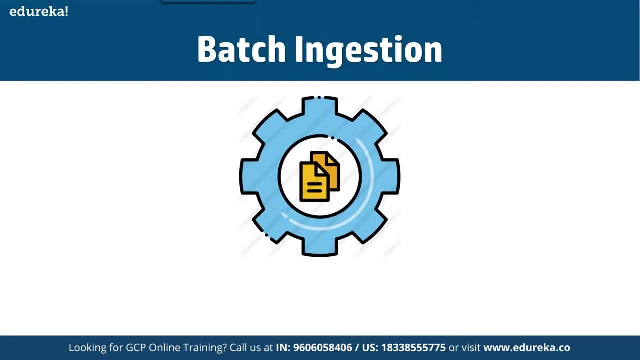 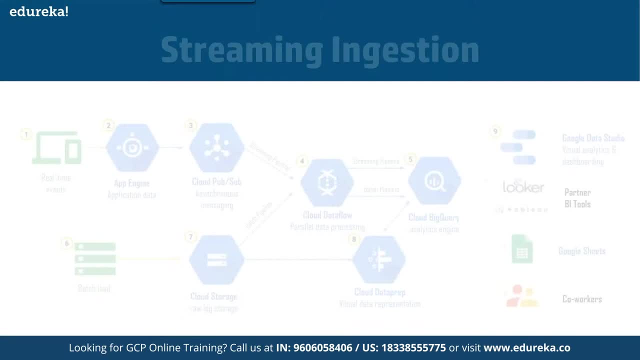 the cell phone it's going to be generated. in the on-premise platform it's going to be appeared together and at the same time it's going to be processed together In the case of streaming ingestion. it's a bit different In the case of streaming ingestion, or you can see in this diagram. 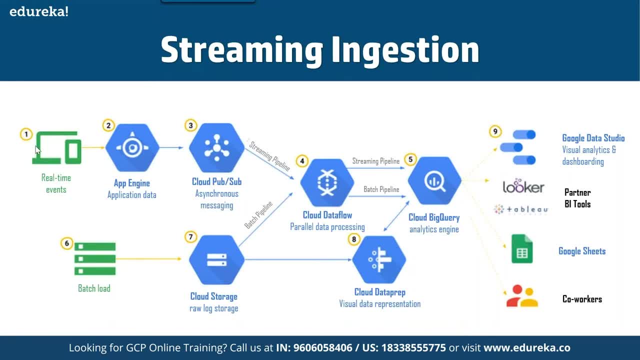 you know you are going to have your real-time events. Maybe I have a service running so it's going to generate real-time events. You are going to have basically the app engine which is going to it with your applications can be on, for mines can be on, a google cloud can be on- uh, you know any? 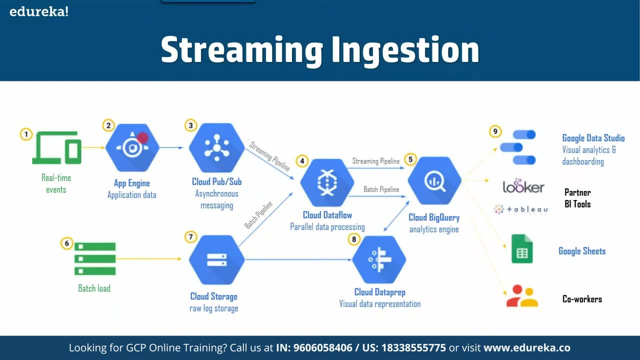 other third-party cloud as well, and uh, these events are going to be, you know, fed together into your uh messaging service. so, any cloud model you talk about- for example, your, you know azure, you have your google or other- they provide the messaging services. so, different type of messaging services, they are provided, with the help of which you can have the request response. 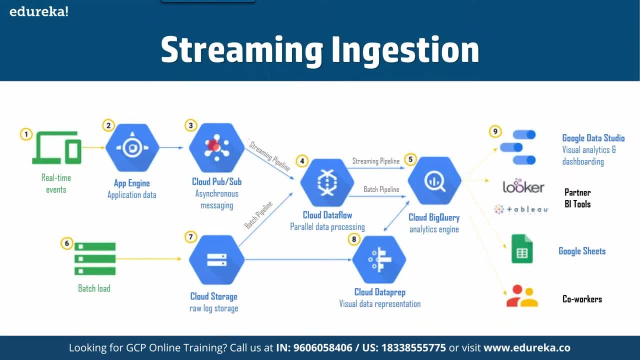 protocol set up, based on which you can also set the acknowledgement. like the way tcp works, you send a request, wait for a response. if there is no response, you send another. uh, you know, same request again, because it will consider that your request has been dropped. so, with the help of stream, 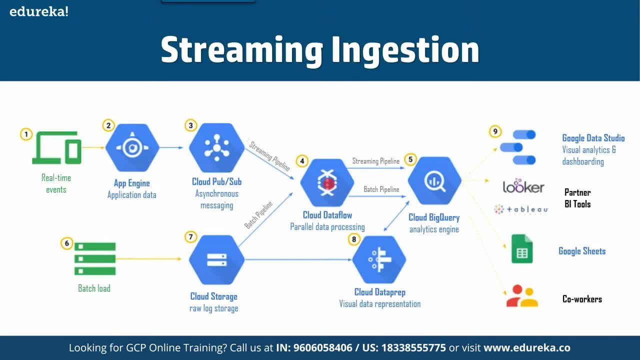 pipeline, the request that you have received is going to be, uh, going to the, you know like, like a queue, where you can have multiple pipelines all together, because it supports parallel communication, and next, when you have a batch pipeline, wherein, uh, you can basically create the batch of cds. 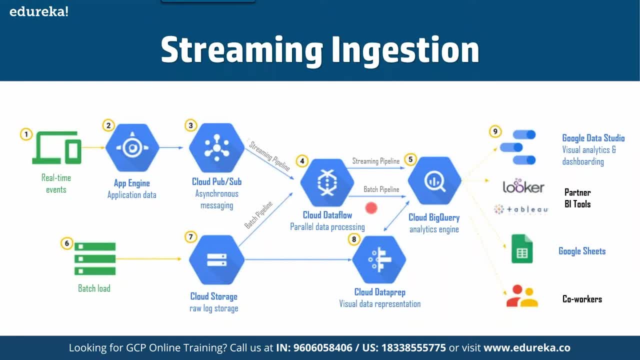 batch of requests which is going to be, you know, accumulated in the queue together and at the end it's going to process together. then after that, uh, you know, you are going to have again- this is a batch processing data which is coming from- you can have a batch load where the requests are accumulated and, uh, you know, at a specific storage. 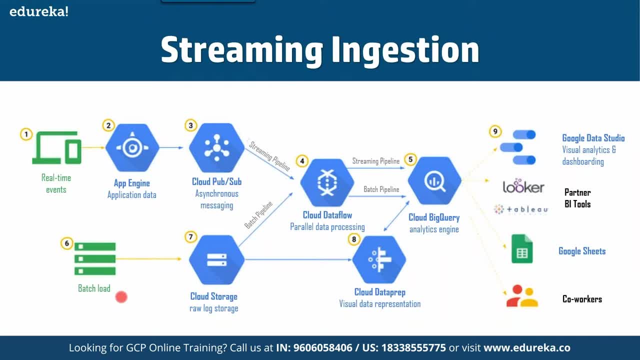 it gets a certain use cases, like your services are running maybe 2 pm every day, 3 pm every day, so it's going to- uh, you know, ingest all the services from different sources to your environment at the same time, which is going to be processed by the cloud data flow and it's going to process together. 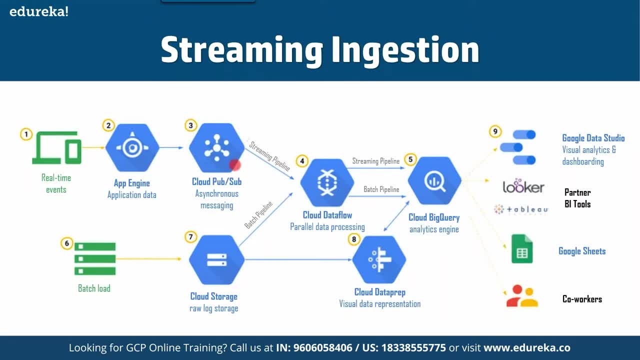 again, this is a very big topic, guys. uh, all three times. uh, we basically have a detailed even this in streaming and ingestion. we basically spend almost an hour on this. however, uh, based on the time constraint that we have, that's why we're just talking about a bit overview of it. otherwise, in general, this is a very big topic. 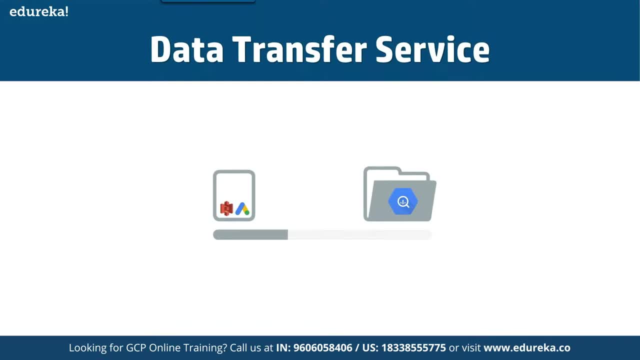 that we cover in detail now. the third service that we have is dts, which is known as data transfer service. so your uh, you know big query- data transfer service is basically a fully managed service to ingest data from your google, uh, sas application. sas is software as service. 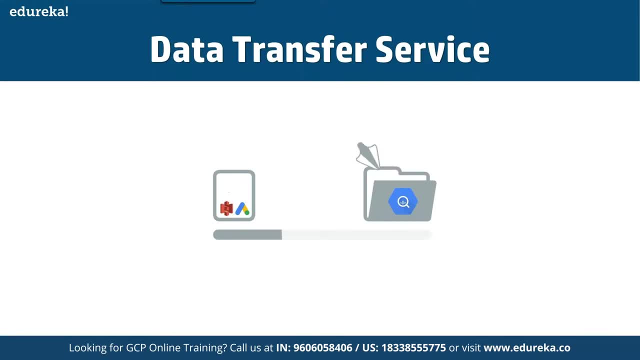 applications like your google ad, your external cloud storage provider, dts, and many other types, so you can transfer data from your dts application, such as your email, like amazon you know on different, different providers we have, and you can transfer the data from data warehouse technologies like your data data, your amazon redshift. so all this thing. 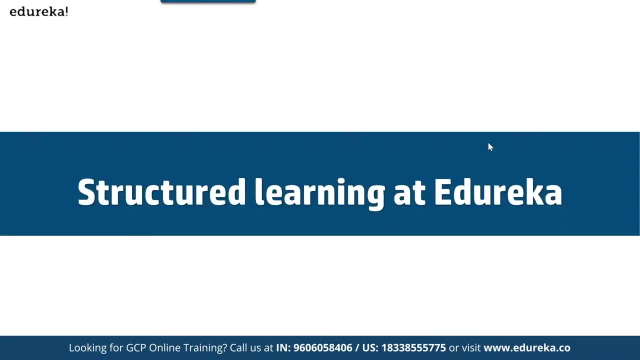 basically falls into this category, which is data transfer service, here and now, in this, now um, coming on to the structure learning editor, aka. so if you want to dive in more detail, you want to enroll for the course and you want to know what all the topics are. like I said, we bring the transferency, so all this kind of topics. 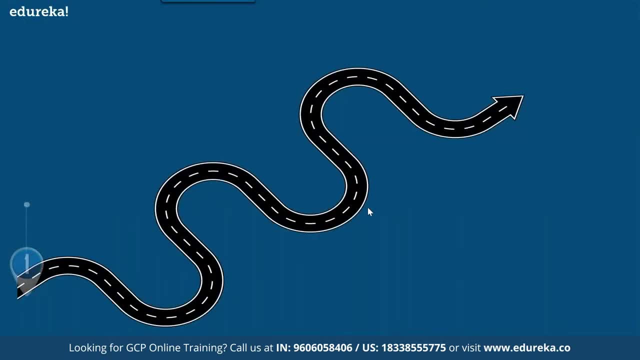 information is available on our website. so let me just share the curve path, the learning path, how it's going to be there. so, if you're going to enroll for the course, this is going to be the learning path. in the first class, you learn about google cloud platform, how you can create. 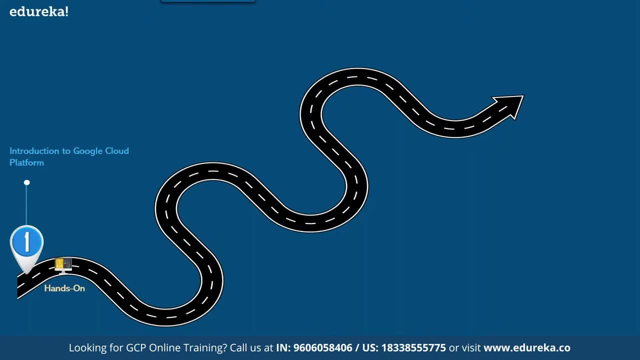 your account, how you can set up the labs, its components, sub components, with the hands-on on different topics. then after that, in the second class, you will learn about how you can basically manage your google platform, its services, its component and sub-components, with the perspective hands-on. then in the third class, you will learn about google cloud platform virtual. 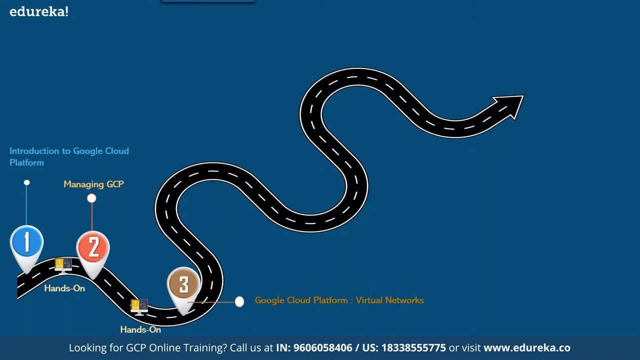 networks, uh, what are different type of networks that you can create with the perspective? and so then in the fourth class you will learn about security and identity fundamentals. um, you know how basically you can create different, different type of access you can. how basically you can control the entire access with you. how basically you can give. 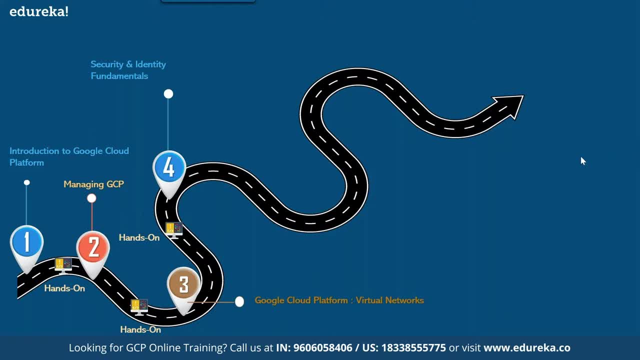 different permissions, how, what are the different roles that you can create, uh. at the same time, you can also or define your own uh, you know, structure like: uh, how many roles you want, how many users you want, because i don't want more than 15 users, you know, to access a resource, so all these kind of things. 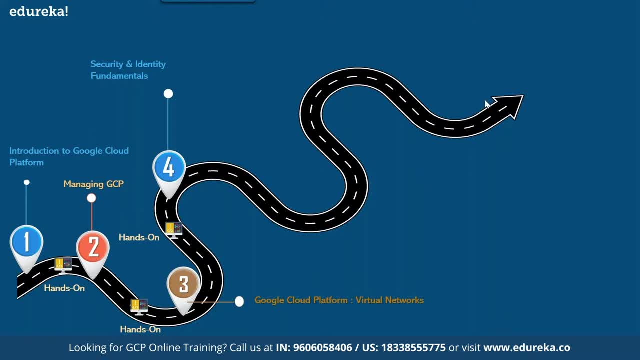 can be restricted uh here that we are going to learn, uh, with practicals, hands-on. then after that you will learn about compute services, different type of storage that you have, different type of, um you know, services, uh that you can leverage, include in the case of cloud, with the practical. 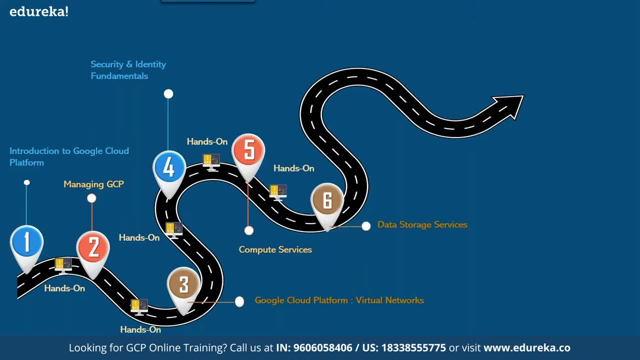 demonstration and the hands-on in the sixth class, you will learn about data storage services. what are different? database that it supports, the different ways of storing it, what are the proprietary of? uh? um, you know google. uh, google has provided, you know, various type of different storage services which it's their own proprietary. what are they? 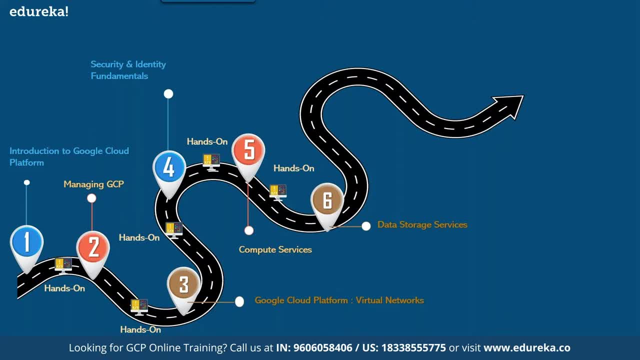 what is the difference between them? uh, how you can select which storage service is based depending on the use case. with the practical hands-on, then in the next class you will learn about architecting with google kubernetes engine. what is docker? what is how you can integrate kubernetes? uh. 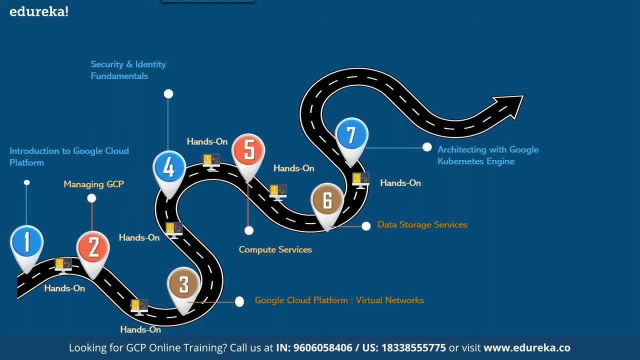 you know how basically kubernetes look like in gcp, how it is different from normal kubernetes, uh, how you can integrate with docker. each and everything you are going to learn in detail with the practical hands-on after that we are going to learn about in the eighth class. you learn about: 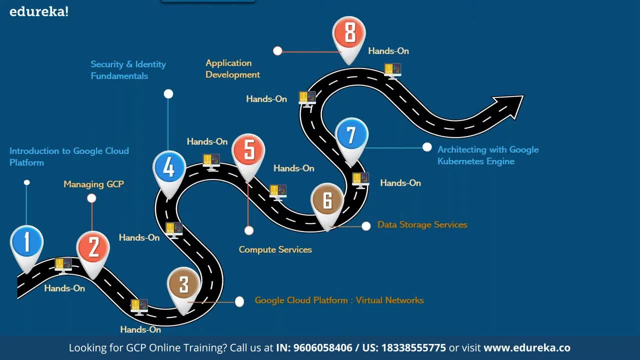 application development. if you don't want to write the code, you want to develop the application. you know how you can do it. it's components of components. with the practical hands-on, then you will learn about big data and ai services and then, in the last class, you will learn how you can perform automation on the components. 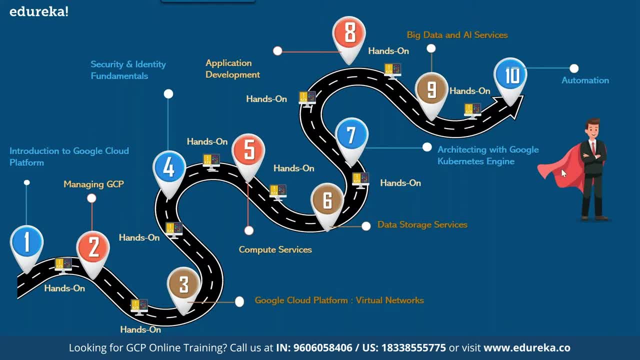 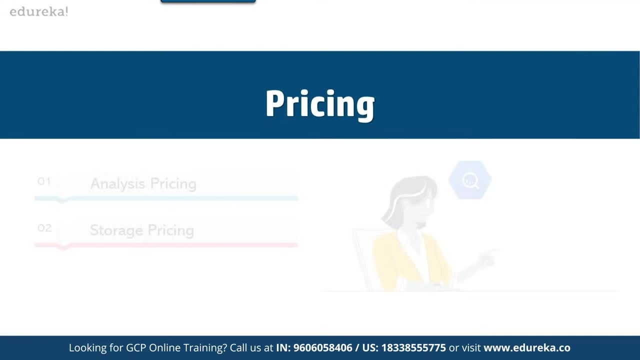 with the practical hands-on. so this is the entire career path, uh, i would say the training path for your certification if you're applying to take. now, coming to the pricing if we talk about, we basically have a two pricing model in the case of, you know, google. that it provides one is analysis. 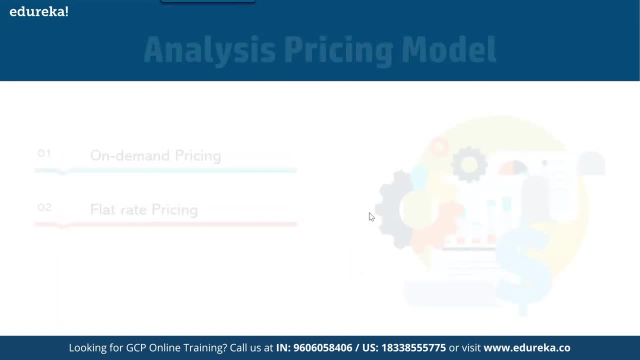 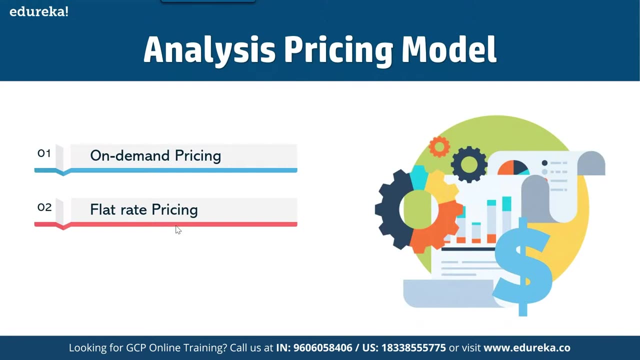 pricing. second is storage pricing. now, if we talk about analysis pricing, this is basically on-demand pricing. uh, basically it has flat rates pricing. in this we have three model. first is you are going to have the annual model. you are going to be basically billed and paid annually. second is on a monthly basis. third, 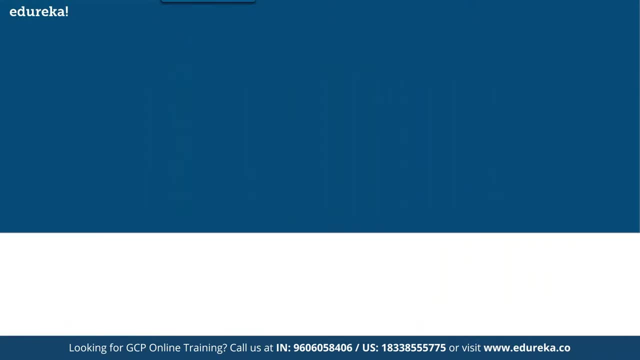 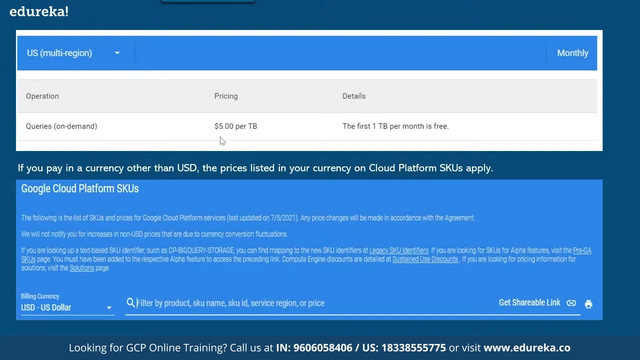 is basically the flexible store slots that you can choose. so this is again one of the example of the pricing model, the way it looks like. for example, queries on demand, you have to pay five dollars per tv. so first tb is going to be free, uh, but after that you have to pay five dollars. 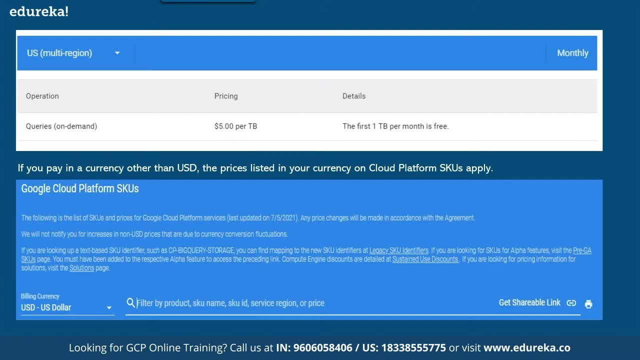 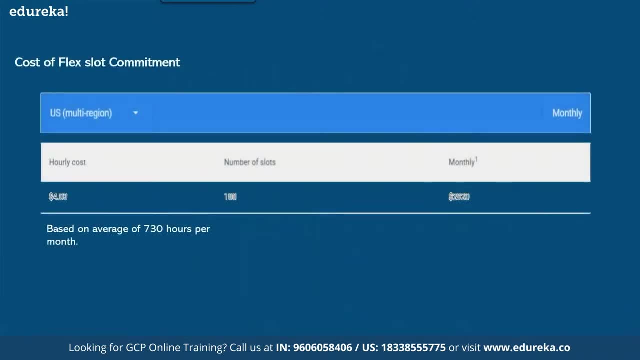 for every tv, which is a you know a good deal as compared to other cloud vendor providers. again, the same thing that i shared a moment ago: a different pricing model that it supports. now, if we talk about the cost of a flexible slot commitment, like i said, we have 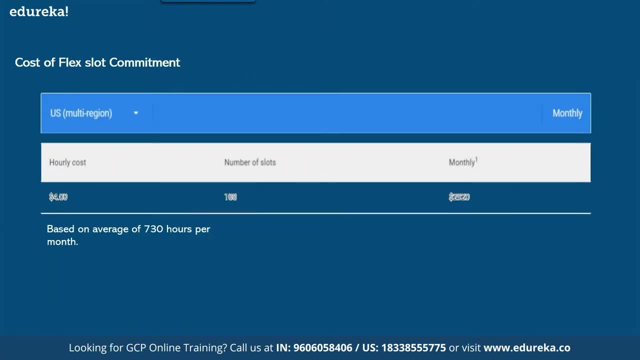 three times the flexible monthly and the annual. so if you, if we basically take a look at flexible slot, you know you're going to get uh, this much slots and uh, you know, based on average of this is 7- 30 hours per month, depending on your requirement. you can decide if you're using. 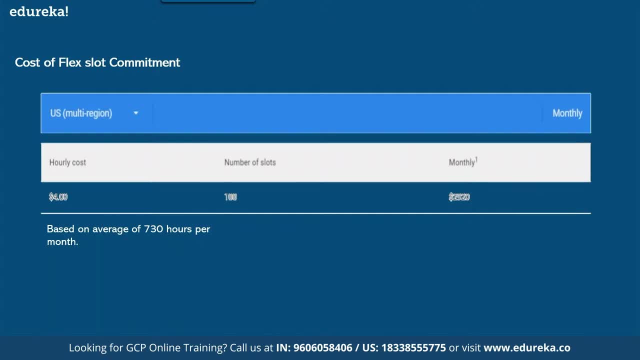 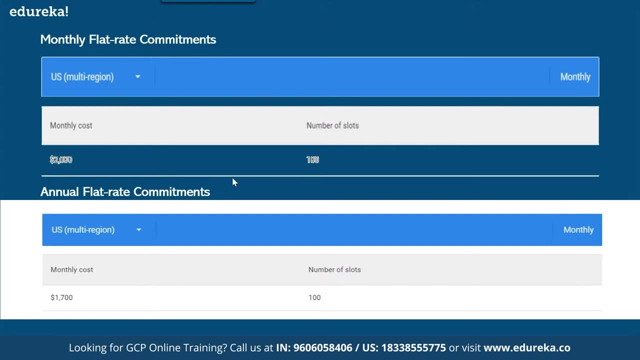 heavily. uh, do you want to go with the flexible or your monthly is going to be a little bit more to be best, or annually is going to be best. likewise, if we talk about, you know, monthly. in the case of monthly number of slots that you get is 100. you have to pay 2 000 for that. in the case, 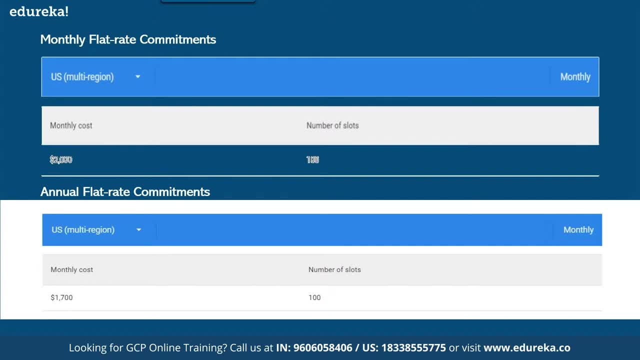 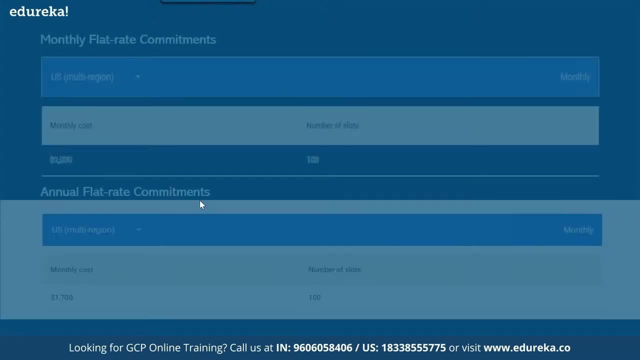 of annually, the amount is less. so where you're going to pay less, which is 1700 now, if you look at the cost in the case of flexi, it's uh, you know a bit more now. you basically look at the cost of your uh monthly. it's high. annually is less, so you can save the money on that now in terms of storage. 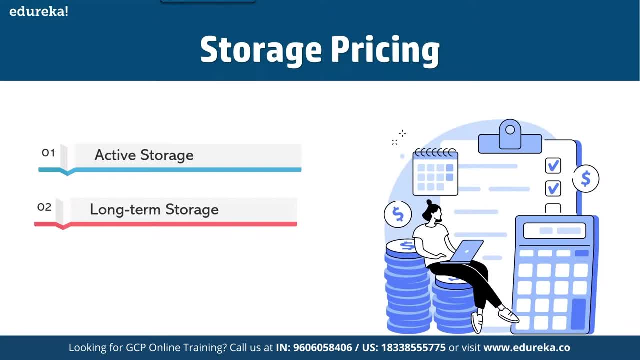 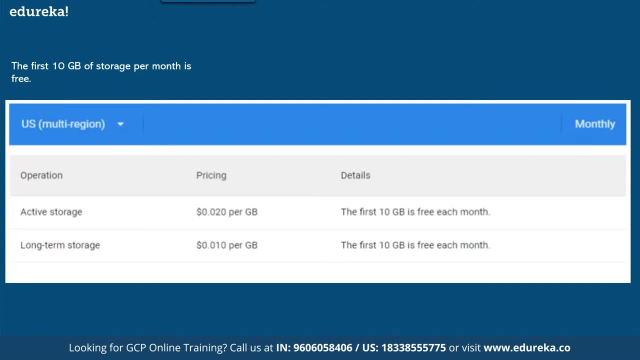 pricing. if you talk about, it has two types of storage pricing. one is external storage pricing- active storage. second is lts, which is long-term storage. so you have seen that, in the case of long-term storage, what will happen? that we even talked about a moment ago, which is which has a 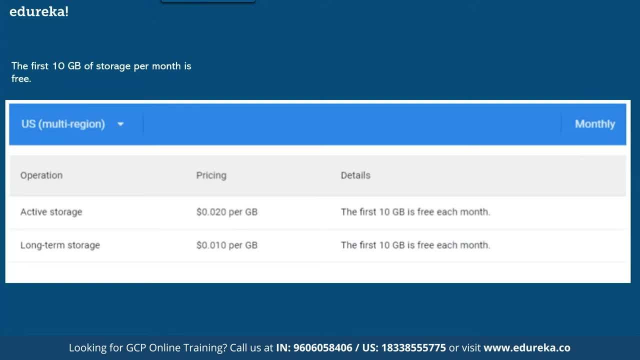 benefit that if your table or partition is not modified for 90 consecutive days, that is going to be considered as a long-term storage and price of that storage is going to be automatically dropped by 50 percent. that's why, in this case, you see, for active storage- uh, it's uh- the cost is 0.02 dollars. 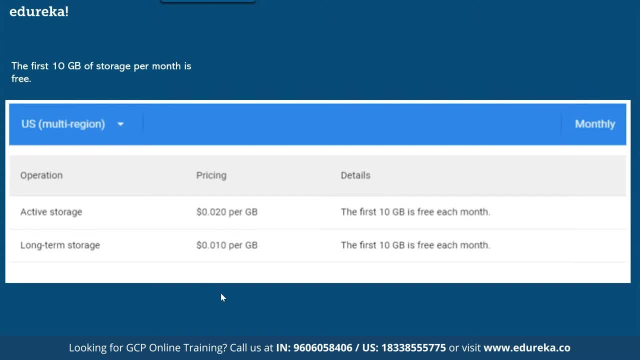 0.02 and for long term it's 0.01, which is half, because the price gets dropped by 50 and in both the cases, the first and gb are free. okay, guys, if we can wrap up for today, it was an immense pleasure to meet all of.